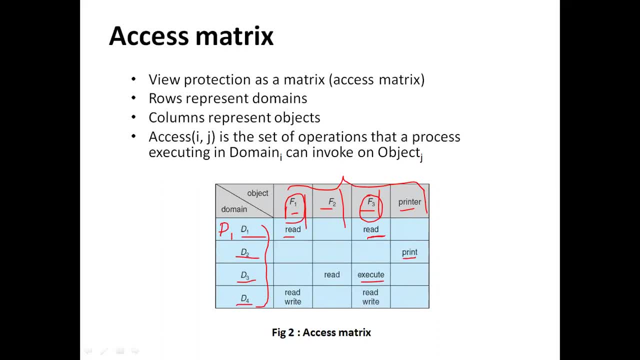 So a process can read F1 or a process can read F3.. Similarly, if this D1 is executing, or any other process for that matter- let's say D1 is executing in domain D2,, then it can only access the printer. It has no other. it has access to no other objects. 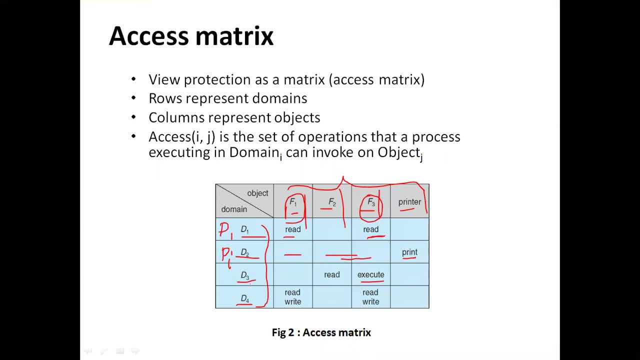 Similarly, if the process is executing in domain D3, then it can execute. sorry, it can access F2 and F3.. So if the process is executing in domain D2, then it can only access the printer. It has no other. it has access to no other objects. 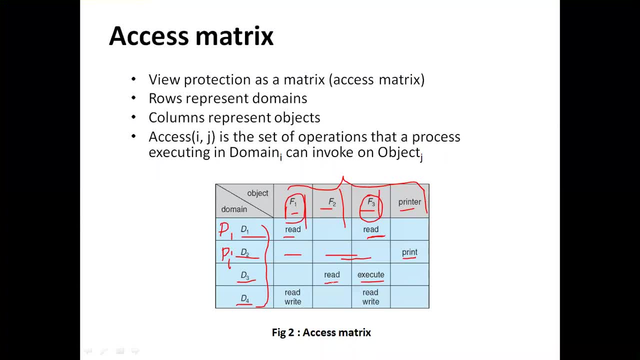 So a process can access F2 and F3 only, and it can read F2 and it can execute F3. That is a process executing in domain D2, can read the file F2 and it can execute the file F3. Similarly, if it is present, if a process is present in domain D4, then it can read and write F1, it can read and write F3. 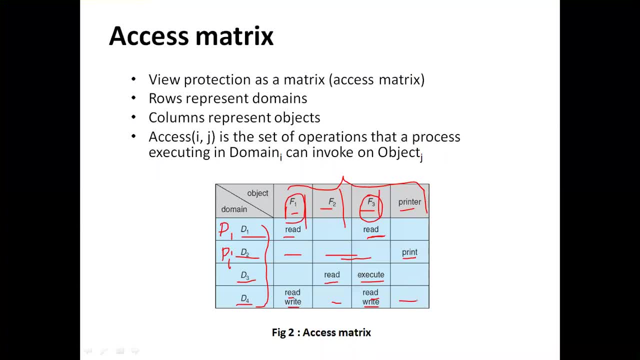 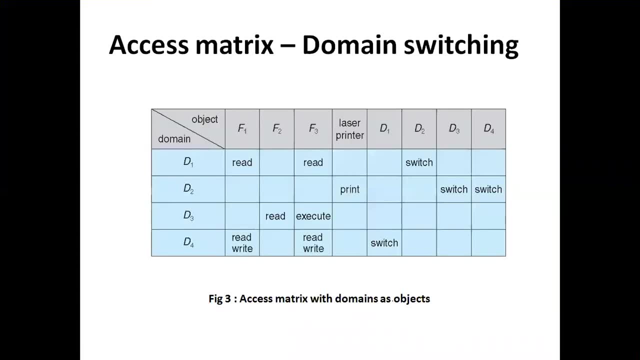 Whereas it cannot access F2, neither can it access a printer. now we have learned about domain switching, so there are times where a process can, a process will have to switch from one domain to another. so this domain switching also can be represented using an access matrix here, along with the resources f1, f2, f3 and a printer. 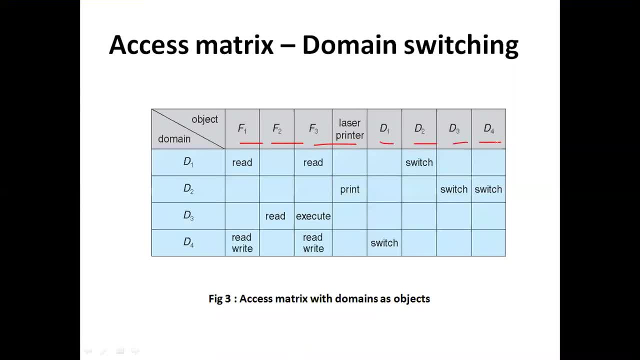 the other domains are also represented as objects of the matrix. so whatever we have here, these columns represent um. so all of these represent objects, whereas these represent domains. we we know that very well. here we have four domains, as it is the. the exact same domains are represented as objects also in the. 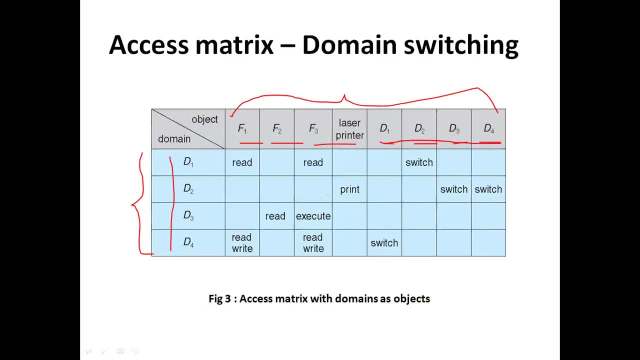 matrix. so this matrix, where you have domains as objects, is required to represent domain switching. now there is an access right now this: read print, execute, write all of these. whatever we have read is an access right. print is an access right, execute is an access right, switch with.